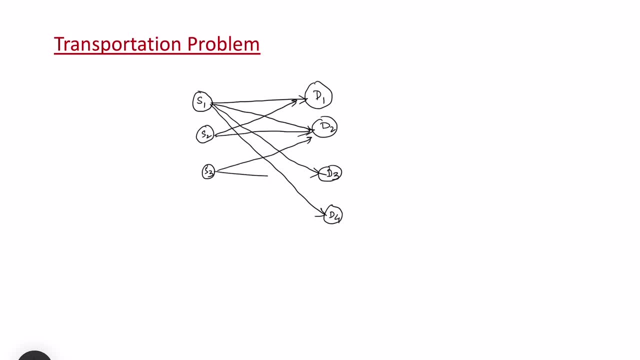 from the other sources. Now it is possible that every source is supplying material to every destination, or it is possible that some of are given restriction that S 3 cannot supply to d4, so this is not supply. so these are called restricted transportation problem. 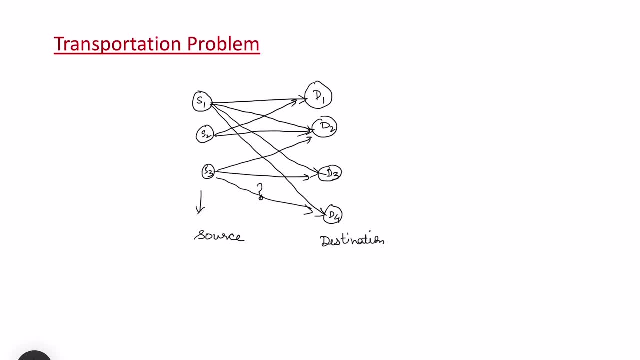 so we'll be discussing both till gradually once we proceed towards this topic. but at this moment i am assuming that this problem is something about the transportation from a particular source to a destination. so let's take an example here. what is the transportation problem to explain this? 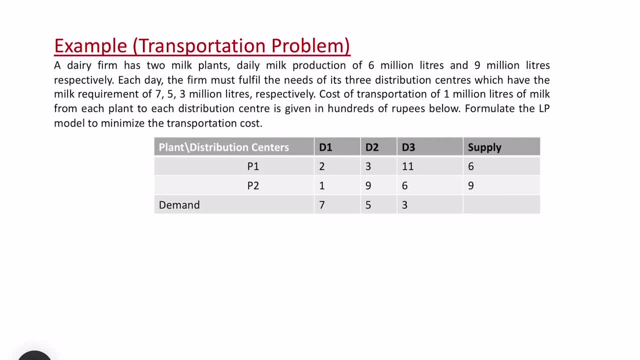 i've just considered a very simple problem. there's a dairy firm which has two milk plant and it has a production of 6 million liters and 9 million liters respectively. so we have considered here the two plants, plant p1 and p2, and then we have certain three distribution centers. 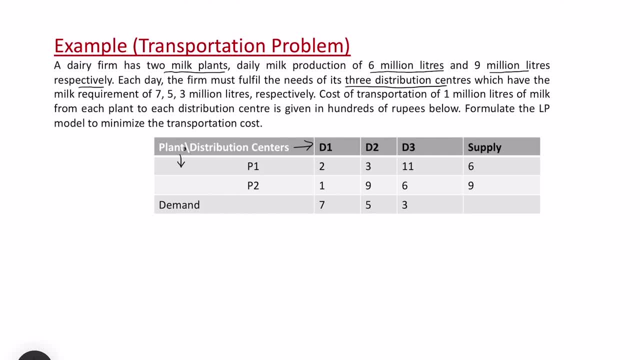 so we have d1, d2, d3 as a distribution center and the milk requirement of these distribution center is 7, 5 and 3 million liters. so that's the demand return here and this is the supply which is given to us as 6. 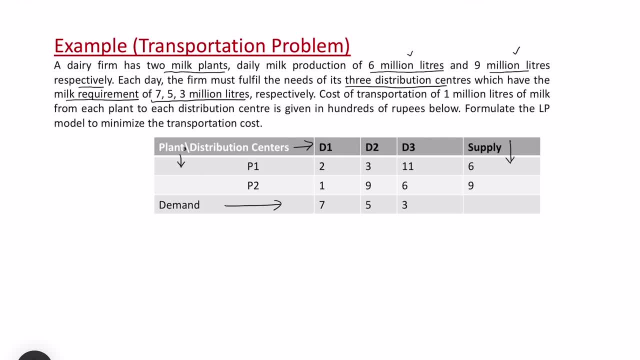 million and 9 million, and here is the demand, return and the cost of transportation of 1 million liter of milk from each plant is given in the table. so this is now at this table. this is the cost of 1 million liters. so 1 million liter here in this question is considered as one unit. 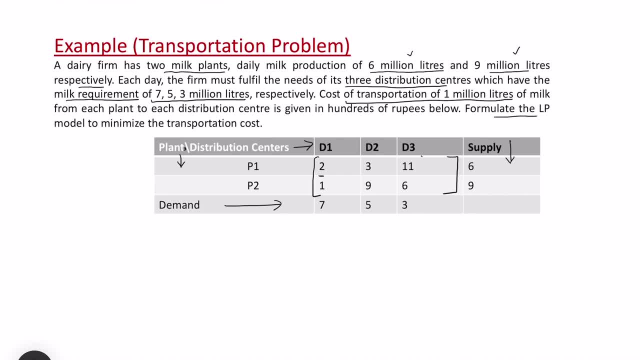 so if we want to now, suppose, formulate this lpp as the minimized transportation cost, we want to formulate now this problem. so what would be the mathematical formulation to this problem? so formulation is: let xij, this be the units of commodity. units of commodity supplied, supplied units of commodity. 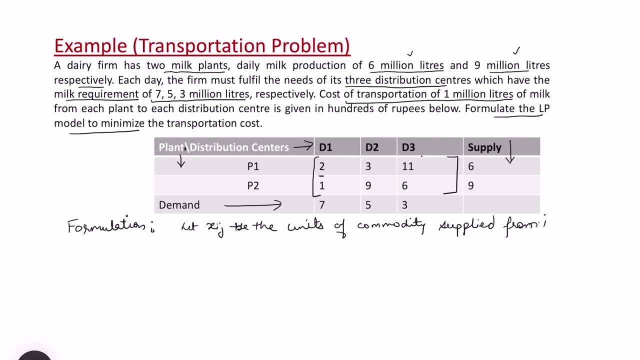 from i'th plant to j'th destination, i'th plant to j'th destination and since there are two plants, so i'll take that i varies from 1 to 2 and there are three destinations, so my j varies from 1 to 3. 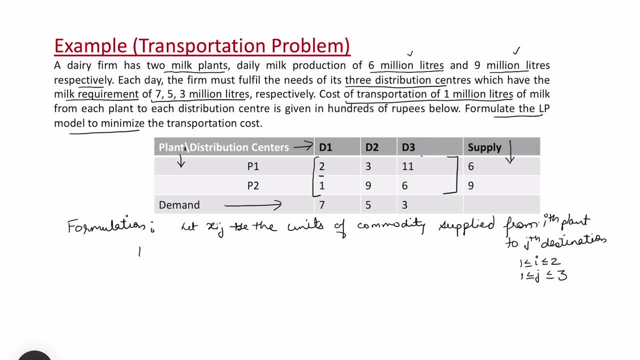 and we want to minimize the total cost. also, the per unit cost is given to us in the table, so that means what is given to us is in the first plant. we have a total cost of 1 million liters, so we want to minimize the total cost of 1 million. 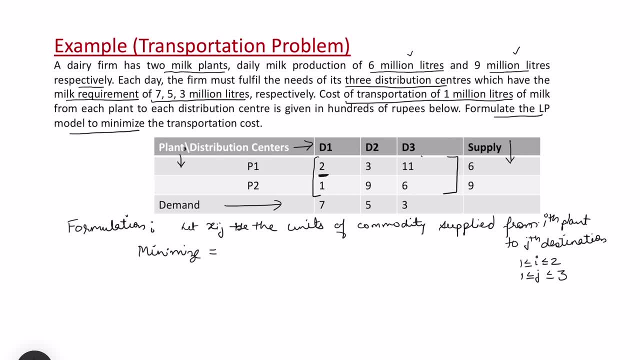 liters. so we want to pot all the particles of materials provided to us for making the m6 plant and first destination this is 2. I am considering this cost in rupees, suppose if it is 2 rupees per 1 million liters. so this means it is 2 times x 11 the number of units which is actually supplied. 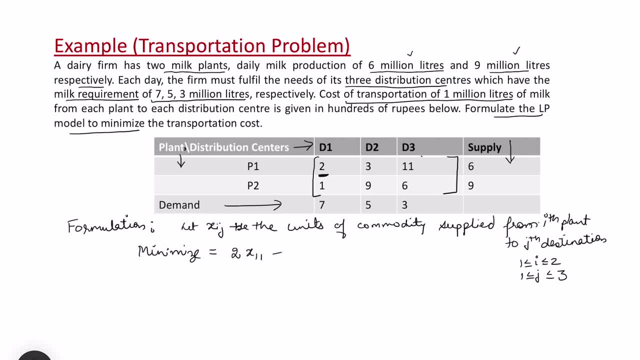 and what was production level, Sweep supplied plus similarly the next quantity at this stage. this is first plan, second destination, so we'll read accordingly and then first plant, third destination. so we have x 1. 3 of this is at two pi, so this is a sub client of two clients. so if one относ to the second line, 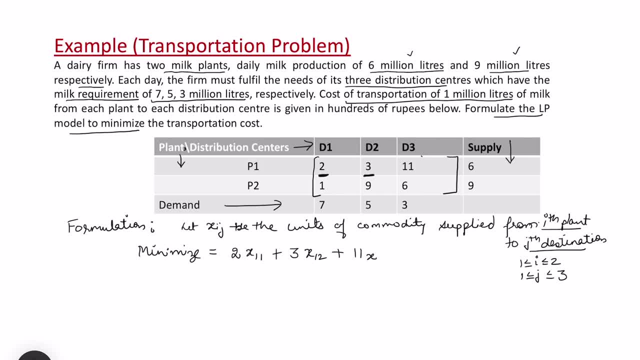 from this at the cost 1 to 3 and the other, so our positive per unit, which is nothing compared to this. so we'll read accordingly and then first plan, third destination: so we have x 13- we want to start planting, and water density, and plus so on. we got x21 plus 9x22, plus 6x23. so that's the cost. this is what we want to minimize. 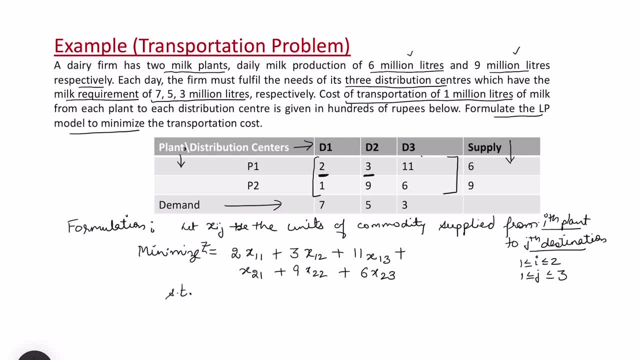 so that's the objective function. condition is that the commodity that we supply. so we have supplied x11 unit here, we have supplied x12 unit here and x13 unit here and on this side we have applied 21- these are the units of the milk that has been transported. so if you sum this one, 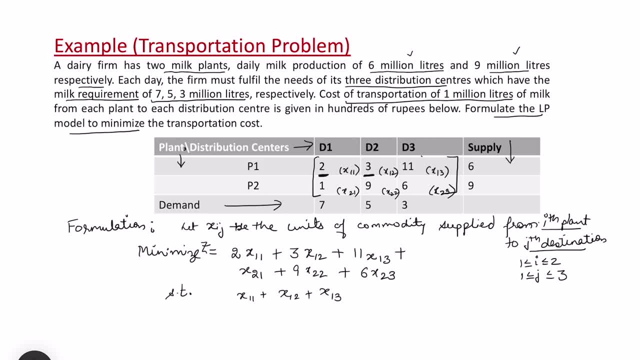 row wise, this is the total number of units of the milk that has available. so this should be always less than or equal to 6, because the supply available is 6 million liter, and similarly for the plant 2. if we consider: for the plant 2, it is x21, 22 plus 23, less than or equal to 9. so this 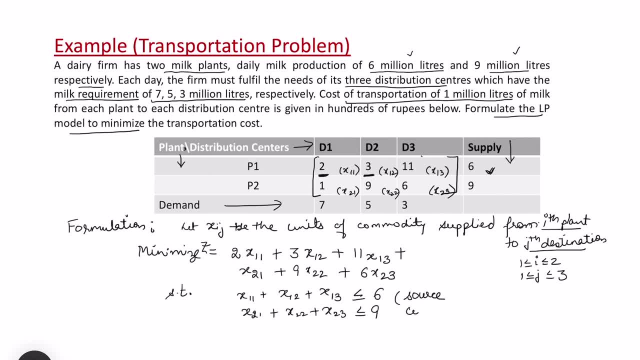 is the total number of units of the milk that has been transported. so if you sum this one row wise, this is what we call source constraint. so they occur because of the source. so these are source constraint, these two. and then we look at column wise. now the destination one is requiring the 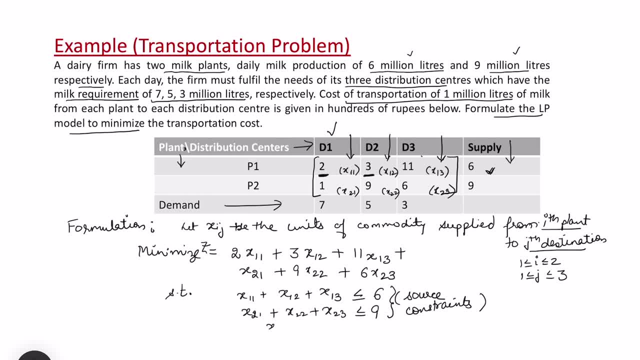 milk from the plant one as well as from the plant two. so this means, if i take x11 plus x21, this should be: the demand should be greater than equal to 7. similarly, x12 plus x22 should be greater than equal to 5, and similarly. 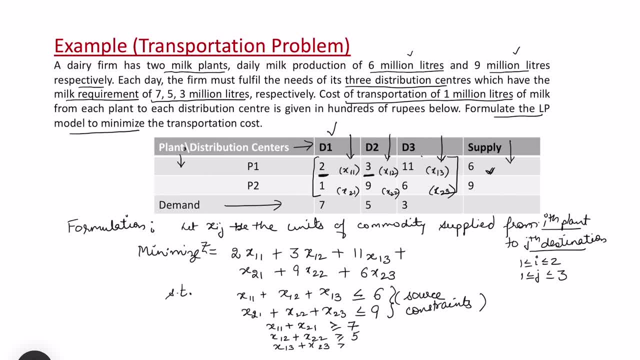 x 1, 3 plus x 2, 3 should be greater than or equal to 3. this is what we called demand constraint, or maybe the expected constraint of the demand. so at this moment i am just calling this as demand constraint, and it is obvious that either the supplied has been done or there is no supply. 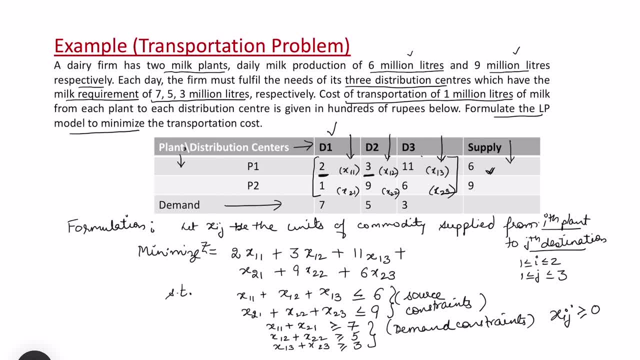 that has been made from ith plant to jth plant. so xij is greater than equal to 0 for all i and j. so this is a simple transportation problem where we have availability and the demand constraint now if you want to look at the general transportation problem. so what will be? 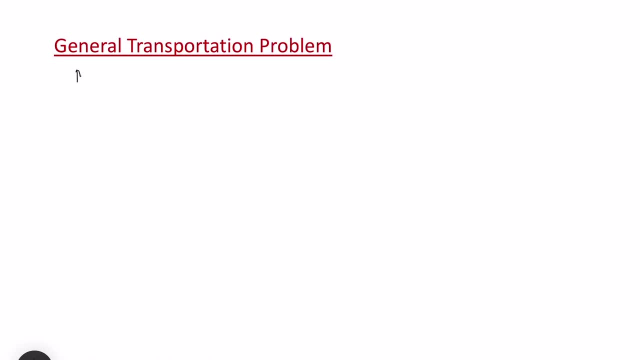 the general transportation problem. so general transportation problem would be actually to minimize z, which is the minimizing the cost of the transportation. so every time if cij is the per unit cost and xij is the total quantity that is supplied, so we sum over i and j, where cij this is per unit cost of ith plant to jth destination. so in the 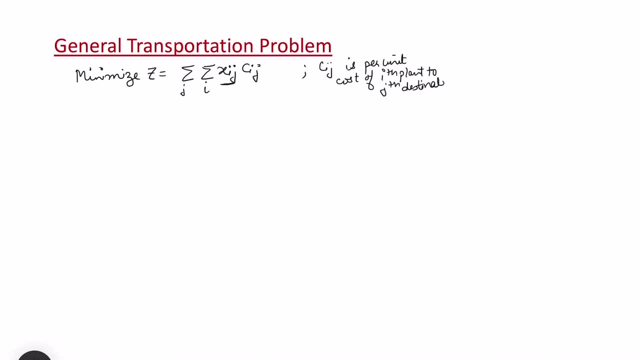 same context, there may be as many as number of plants and there may be as many as number of plant or sources, whatever we want to call this as, and xij. this is the units of commodity transported. units of commodity transported. okay, and subject to now, if we subject in this, in the 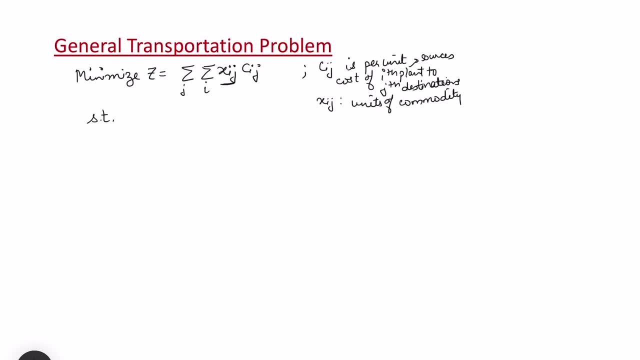 view of the last example, if we sum it row wise, so i am taking it as x11, x12, suppose i varies from 1 to m. there are m number of sources and then there are n number of destinations, so there is a problem here. i am just considering that we have total m number of sources. 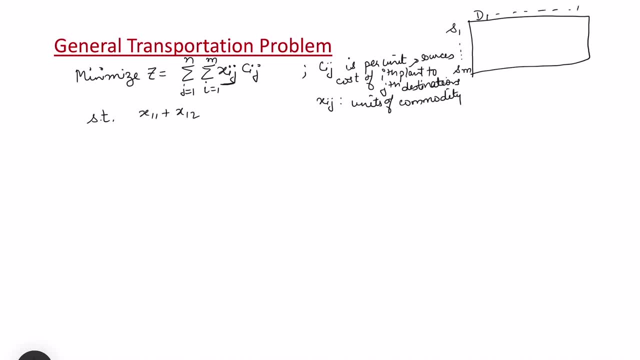 and this demand is n number of destination. in this case i varies from 1 to m because we have considered m number of sources and we have considered j number of destination. so in this case that means there would be till 1n and it is less than or equal, to suppose the supply is a1. 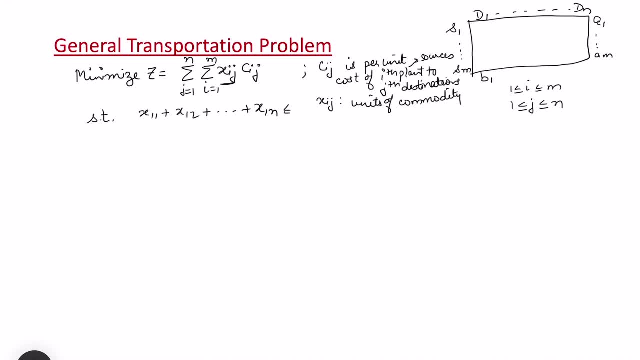 and here it is, am. and similarly, the demand is b1, b2, up till bn, so this is less than or equal to a1. and then similarly, 21 plus x22, plus, so on, plus x2n, less than or equal to a2. and in the similar approach, i am writing the last constraint, mth constraint. 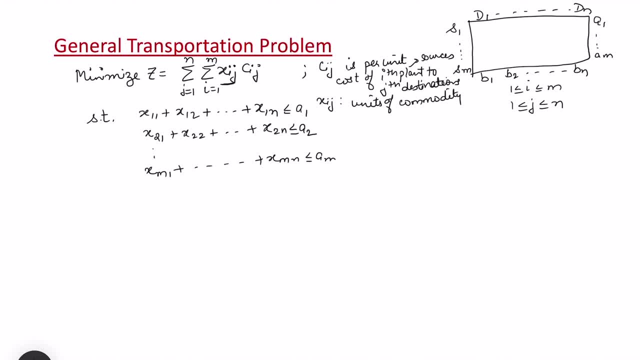 this is less than or equal to am. so this is what we call source constraint. so in general and similarly, if we now sum the column wise, if we now sum the variable column, so in when we sum it column wise, it is the first variable, then second row, first variable, and so on. 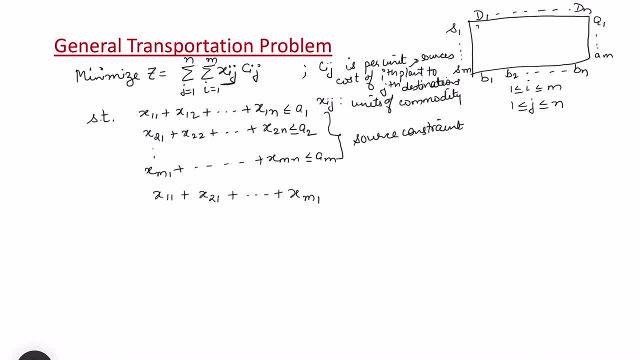 and xm1, because there are m number of variables. so here we may have x11 till x1n. this was xm1 till xmn, so in total we had mn variable and since this is demand, so this is greater than equal to b1 and so on. so the last constraint here is 1n. 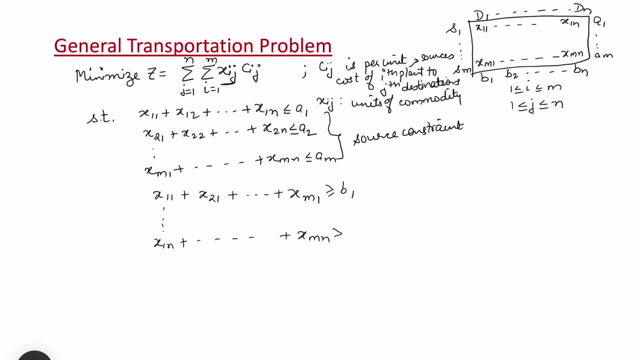 up till xn, xmn greater than or equal to bn, and this is what we called as in the last case, this is what we call demand constraint, demand constraints. and xij should be greater than equal to 0. so now this is what is in the written in the very expanded form. sometime we may write this in a very closed. 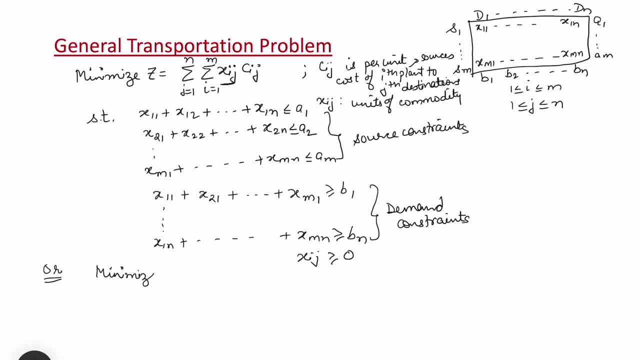 form. so i may write this lpp, because we see here objective function is linear and the constraint are linear, so it is actually a particular case of linear programming problem only. so here i am writing this in a very, very closed form. i varying from 1 to m, j varying from 1 to n. now look at the first constraint. 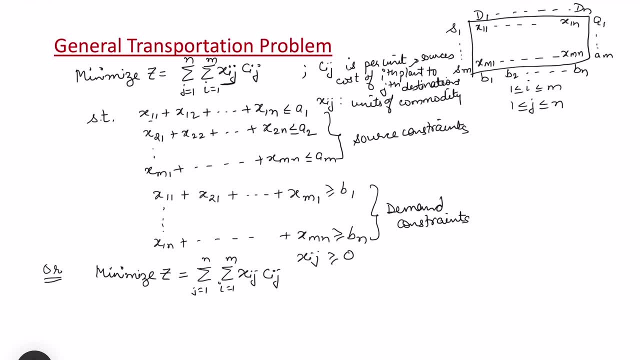 very carefully. the first constraint means the first index, 1, it is fixed, and the second index is varying 1 to n. so this means it is summation xij. j varies from 1 to n. it is less than or equal to ai. so if you keep on substituting i. 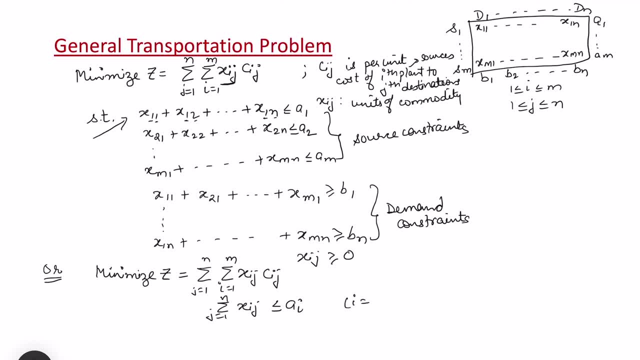 equal to 1, you get first constraint. if you take i is equal to 2, you get second constraint, you and so on. so i varying from 1 to m. so this is how we can write all these constraints which are source constraint, as in this one constraint and similarly. so this is what is. 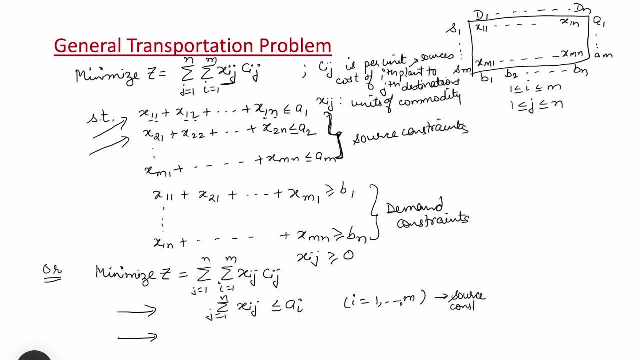 my source constraint and similarly we can have summation i varying from 1 to m. now in this demand constraint we see that i is equal to 1 and i is less than or equal to n. so if we have a demand constraint, we see here now i th variable is moving 1 to up till m. so 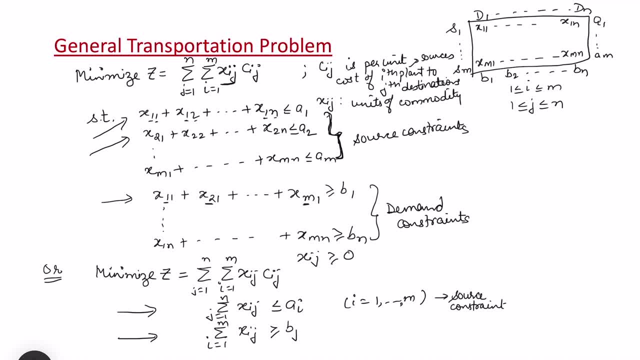 this is xij greater than or equal to bj, and xij is greater than equal to 0. so this is the general transportation problem. but while solving these transportation problem, we always consider the equality in the constraint, so equality in the resource constraint and equality in the demand constraint. 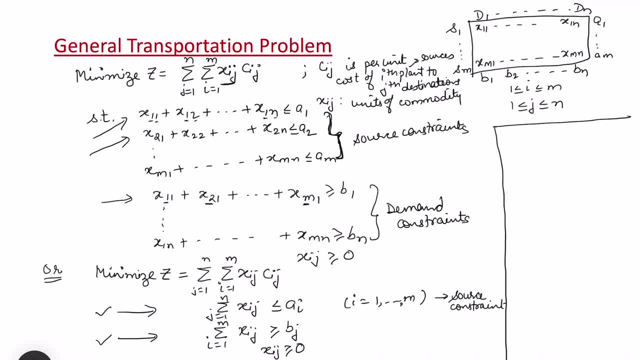 So we consider A constraint A constraint. So we find off a standard transportation problem, standard transportation problem. so what is standard transportation problem in the same transportation? i am going to consider minimum xij, cij. summation over i, summation over j. subject to summation over xij equal to ai. 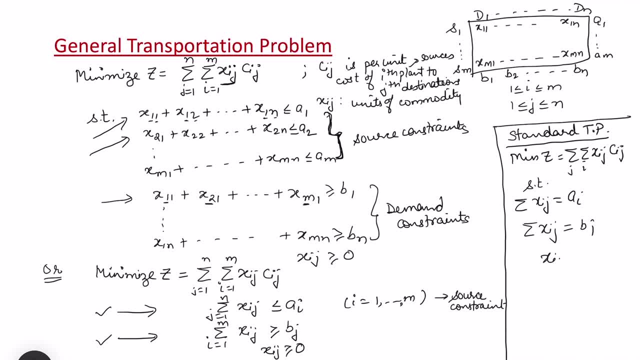 summation over xij equal to bj and xij is greater than or equal to 0, so this is the standard transport. we always know how to convert the constraint inequality. we can always have the physical meaning associated here, because when we have here less than and greater than, so we can introduce the 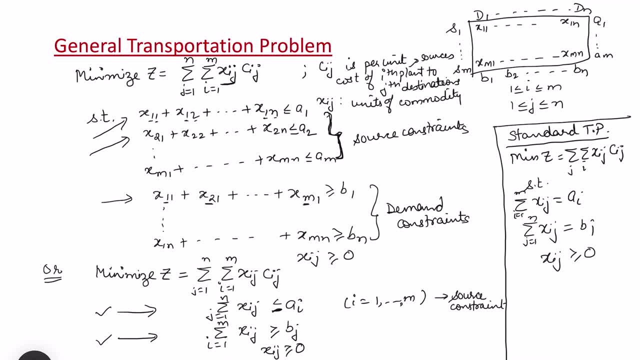 slag and surplus variable accordingly, but still they have some physical meaning about the supply and demand. but in a simple way, i'm just considering that we consider here the standard transportation problem with an equality system. now, with this equality system and also another point that i want to make here is, although we start the transportation problem by minimizing the cost, 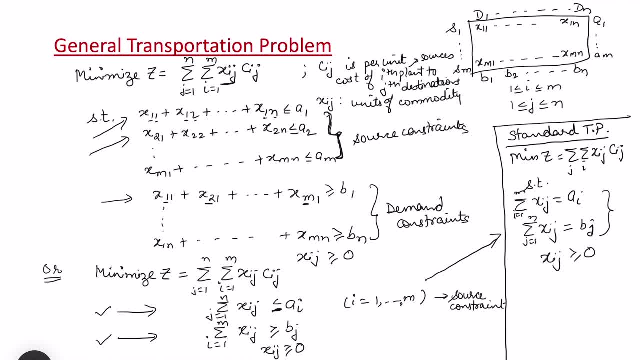 that we want to minimize the cost of supply from the resources to destination. but if we think from a business point of view- and i have a transportation business- i want to maximize my profit if this is given as, if this is given as a, so transportation problem can be. 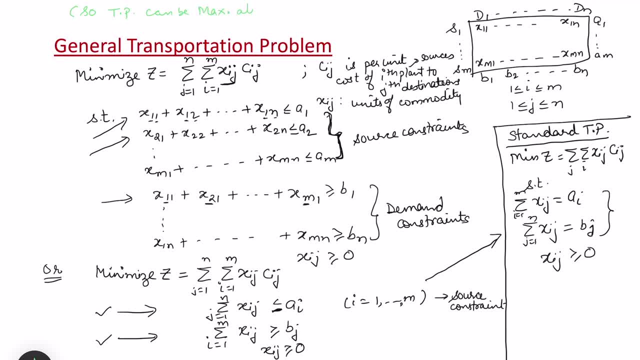 a maximization also. so in the similar manner we can have a maximization of z equal to summation x, ij, c ij. in that case this c ij is a profit per unit in each route. suppose if there is a supply from s1 to d1. so per unit we get c ij as the profit and whatever total number of unit we are sending. 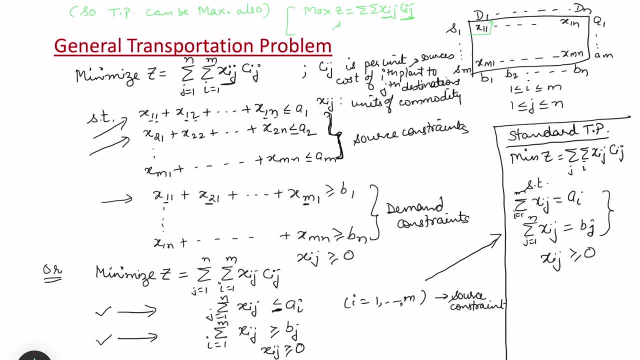 this is multiplied by this x? ij subject to now. now constraint has nothing to do with the profit or the cost, so the constraint remains same, that x? ij is equal to a in the standard form and this remains as bj. x ij greater than equal to 0. 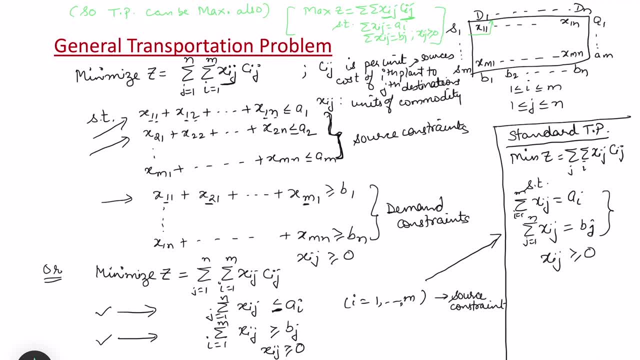 but mostly in the practical situation, we always want to minimize the transportation cost. so the solution that we are going to discuss in coming videos is keeping in mind that we are solving a minimization transportation problem and not the maximization. but in case we want to find a solution for maximization problem, then we can convert this maximization problem into 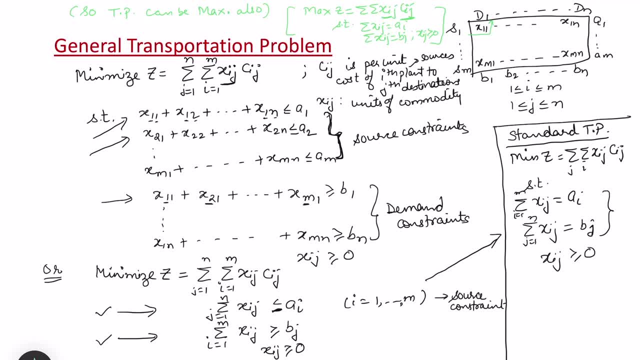 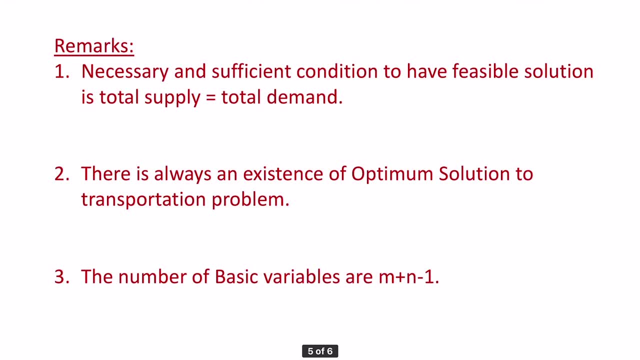 minimization, or we may even directly solve that. so now let's see further. there are three very, very important remark that we need to first prove necessary and sufficient condition to have feasible solution is: the total supply is equal to total demand. so that's a very important condition that we need to take before solving the question. 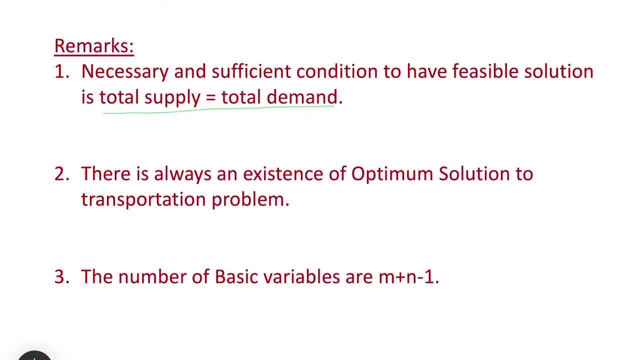 and if this condition holds, then we say that the transportation problem, this is balanced transportation problem. if this condition- so here the total supply, because supply, i have denoted it by ai's and the total demand, i have denoted it by bj, if this hold, if the two are equal, then i'm 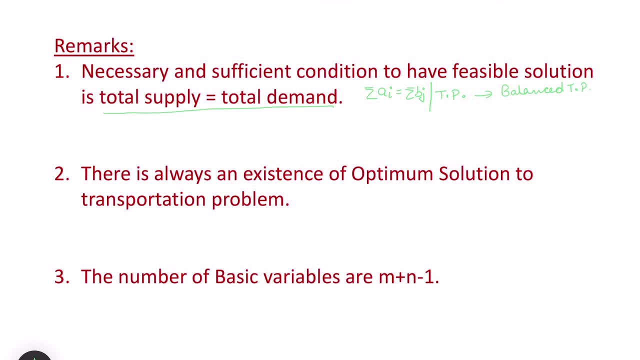 calling time time, transportation problem as balanced transportation problem. and if summation of ai supply is not equal to demand, then transportation problem. we may call this as unbalanced transportation problem. now, every time we solve our problem, it has to be balanced. if it is not balanced, or if it is,